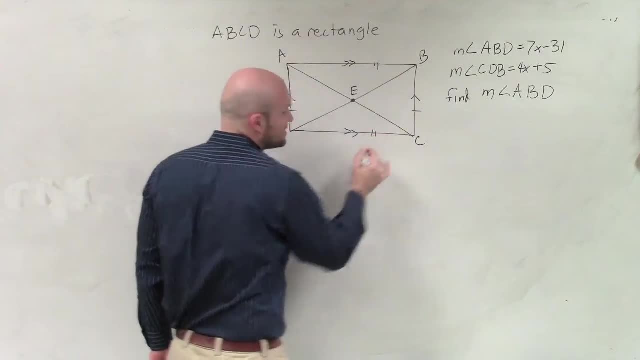 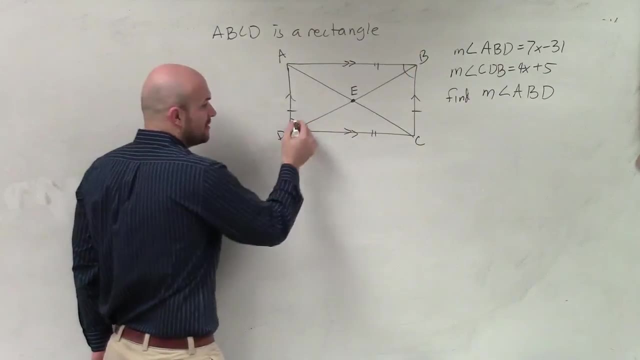 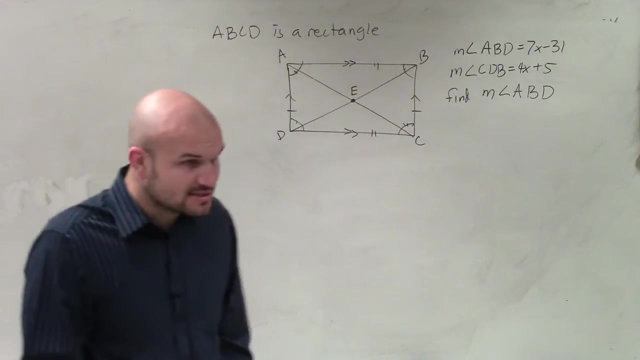 We also have opposite sides that are congruent. These are all parts of being a parallelogram. We also have opposite angles that are congruent, right? Those two are equal to each other And these two angles are equal to each other. That's a part of being a parallelogram, right? Those are all qualities of a parallelogram We all need to know by this point. 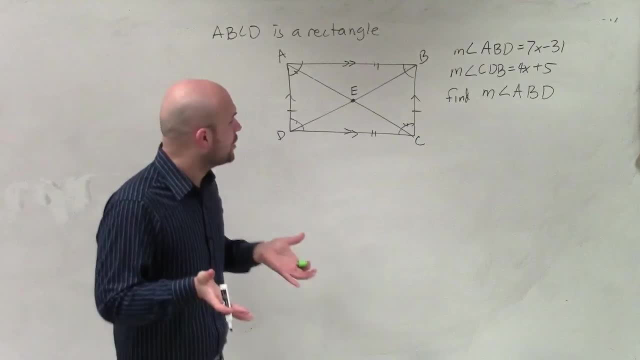 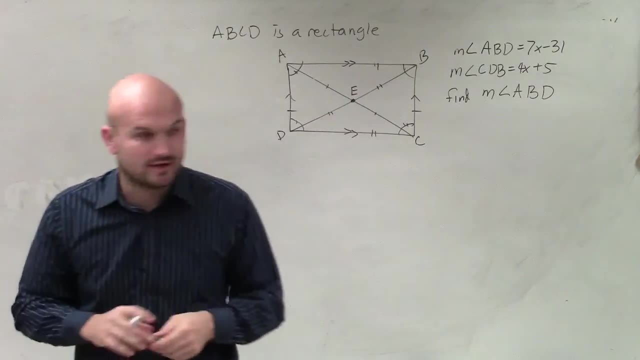 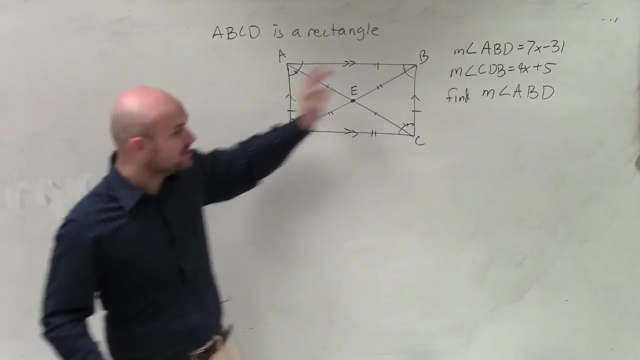 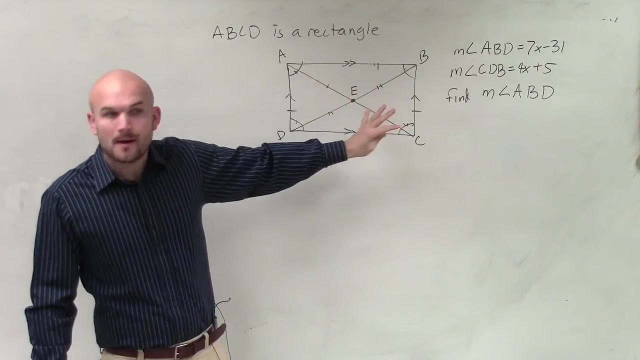 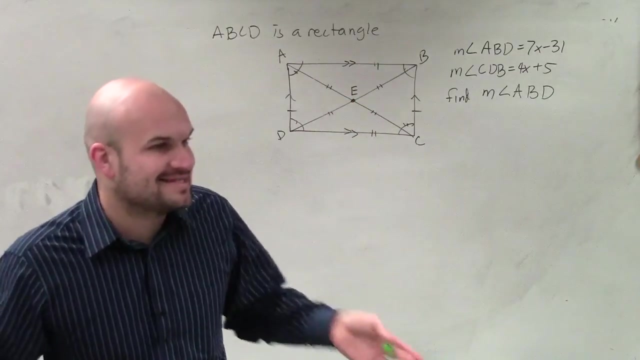 Then the next thing we talk about is rectangles. Well, how are rectangles? also, as far as a parallelogram, that we know that these bisectors, They bisect each other. right, Your diagonals bisect each other. That's another quality of a parallelogram. But now we're talking about a rectangle And a rectangle. what was important about a rectangle is: all these qualities are true, except now there's a couple little differences. Yes, the diagonals bisect each other, but now the diagonals are also equal in measurement. right, The diagonals have the exact same measurement. 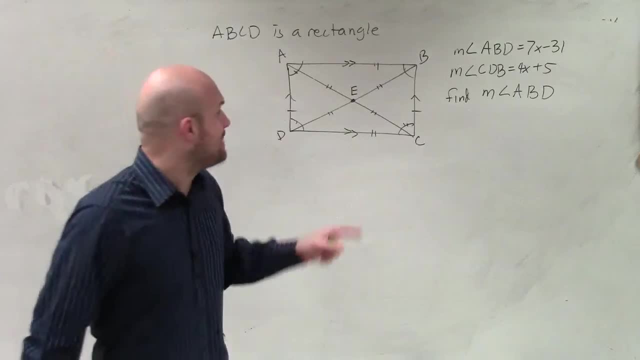 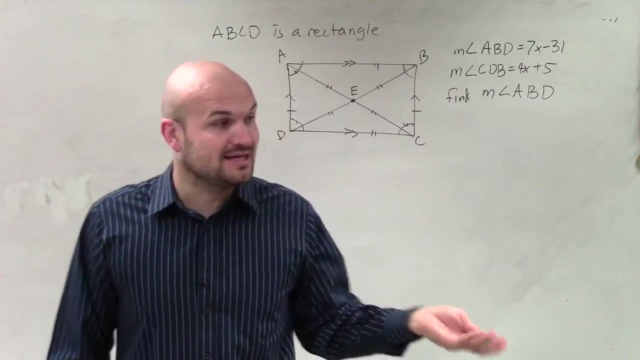 Diagonals have the exact same measurement, So when they bisect each other, that means all these lengths are equal. Opposite angles are exactly equal to each other. but, Mario, what are now the angle measurements? What do we know about the angle measurements of a rectangle? 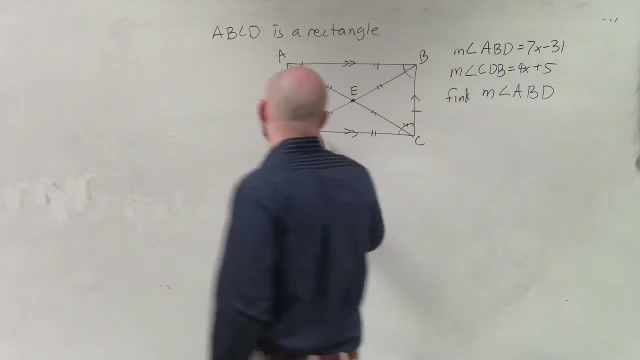 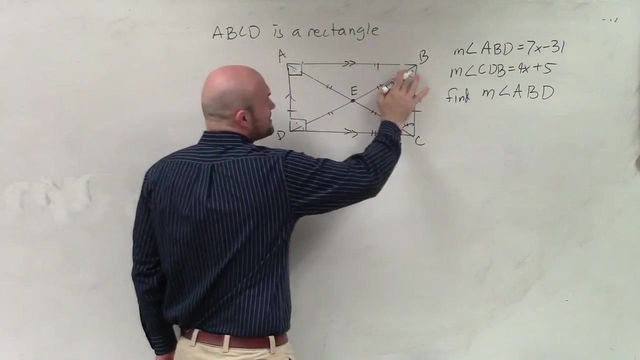 Every angle is 90 degrees. That's a right angle, So I don't need to draw these little arcs. I can draw now the boxes Because, yes, opposite angles are equal, but now I know that the measure is 90 degrees. 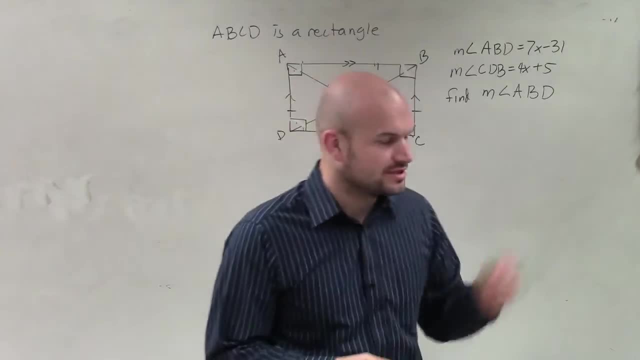 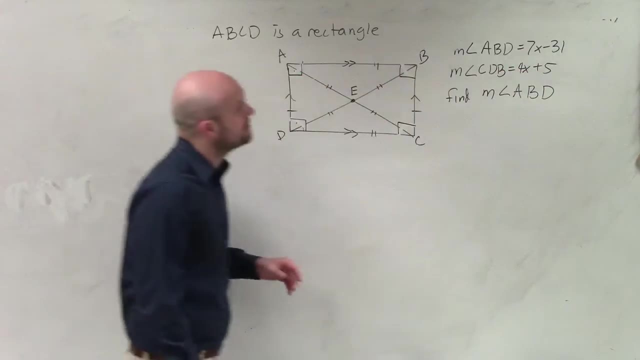 All right, So now let's get into what the question good, gentlemen. So now let's go and get into what the question is asking for. this problem, In this problem, the question says the measure: do you need this or not? 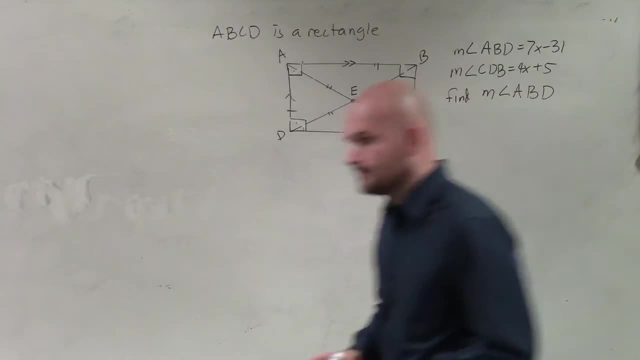 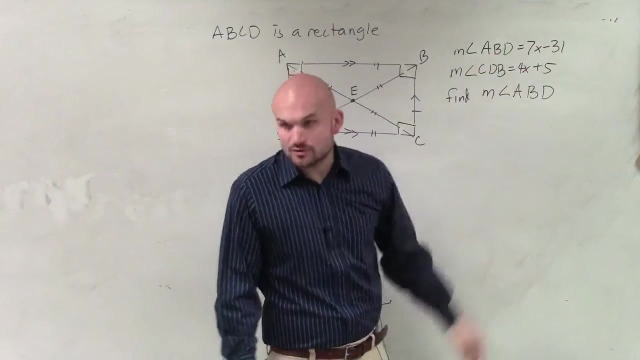 Yeah, Okay, No, it's just a device. Oh, okay, I'll give it to him. Thank you, Pass it back, please. So now the problem is saying: measure of angle ABD is equal to 7X minus 31.. So again, let's find ABD. 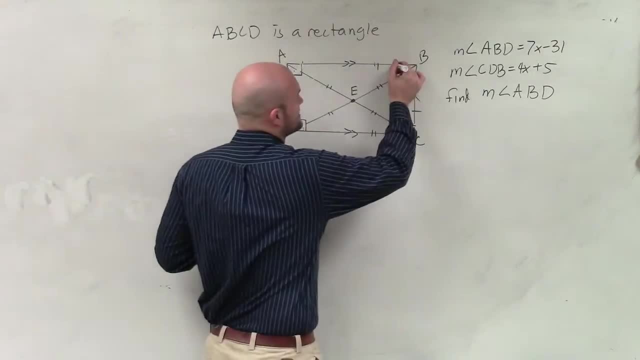 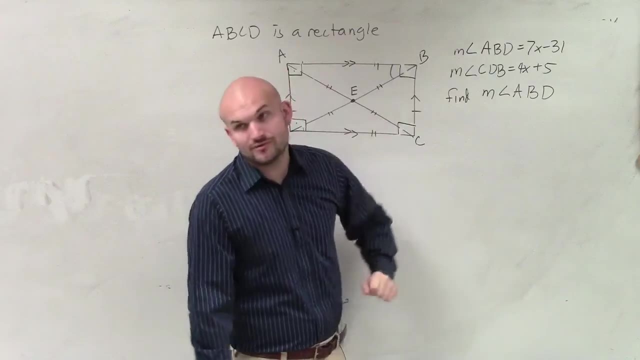 A, B to D. That's right there. Okay, That is equal to 7X minus 31.. Then it says measure of CDB is equal to 4X plus 5.. C, was that right? Did I write those in there right? 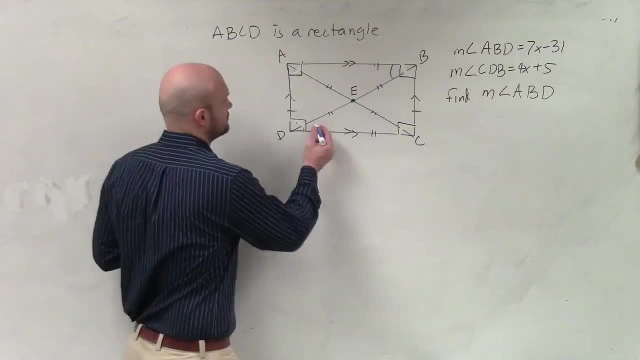 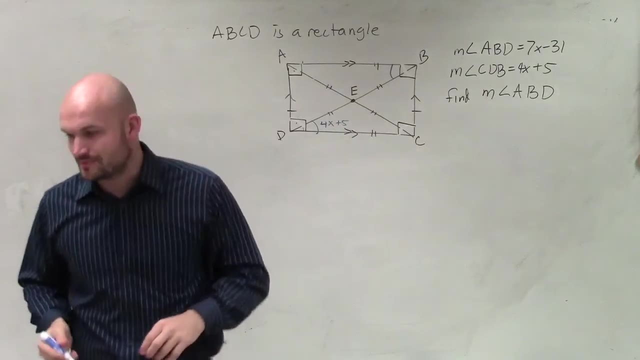 Okay, C, D to B. I guess you guys didn't do them. I guess you guys did do it right, I'm sorry. 4X plus 5.. I guess I looked at the problem wrong. So now we need to say: all right, find the measure of ABD. 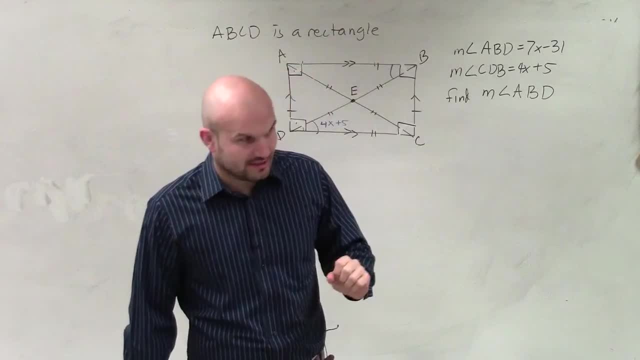 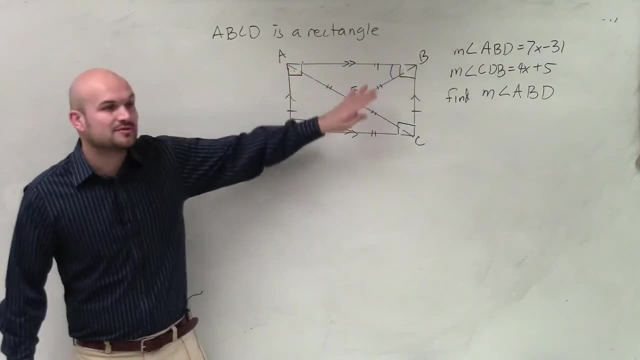 Well before we can even find the measure of ABD. Oscar, this will be your second last time warning. Okay, That needs to be flipped down. No, flipped over down. Okay, So now what we need to do is be able to find the value of X. 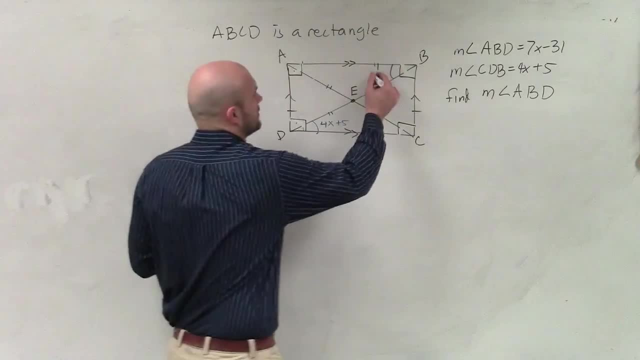 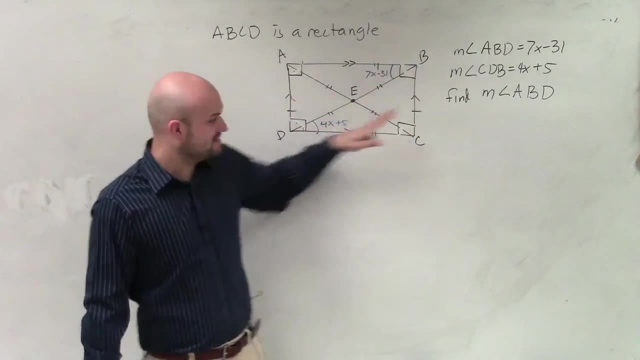 So we look at how are these two related to each other? And one thing that's important about knowing a rectangle is a parallelogram, since these are parallel lines and we have a line that's cutting through them, which we call a transverse. 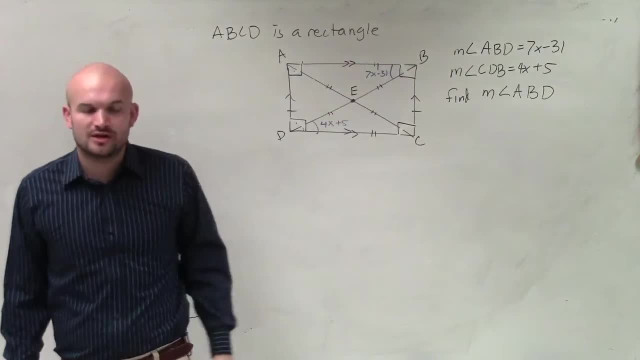 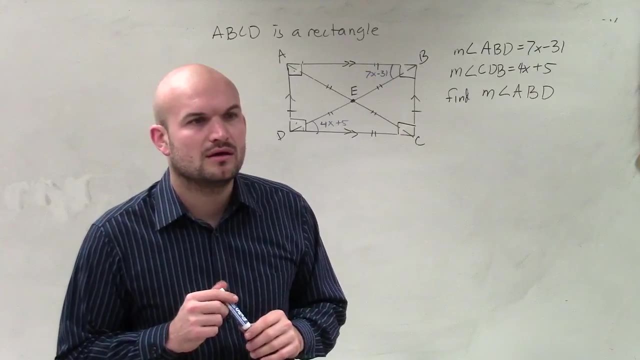 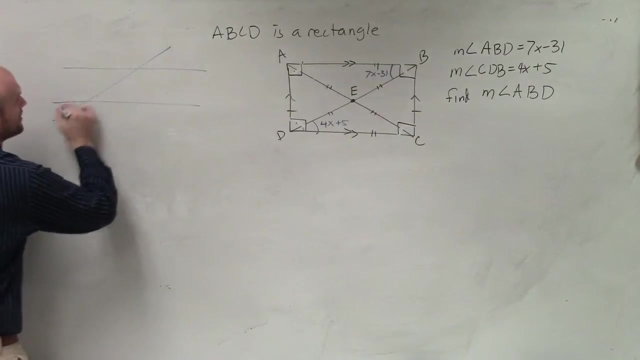 we could say that these two angles are equal to each other. but, Zach, why would you say they're equal to each other? What angle relationship would you say those two angles have If I was to draw parallel lines and I was going to say this angle and that angle? 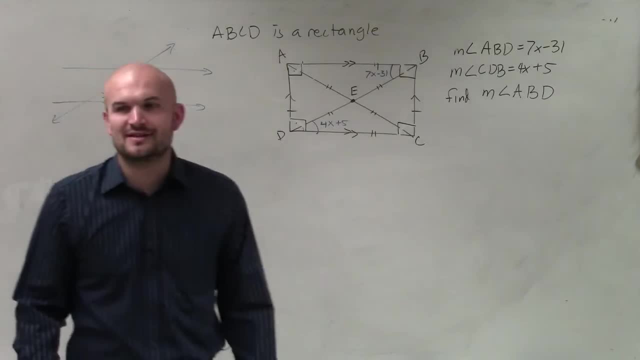 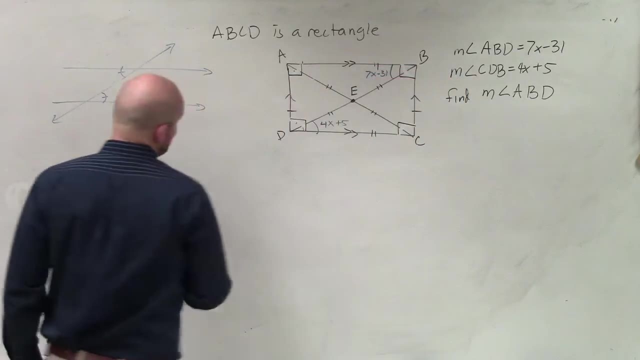 yeah, not opposite interior, but what's another way for saying things are on the opposite side of the transversal? Yes, Blake, Alternate, Alternate interior, right? So these are alternate interior which are equal to each other. So therefore, you can say: 7X minus 31 equals 4X plus 5.. 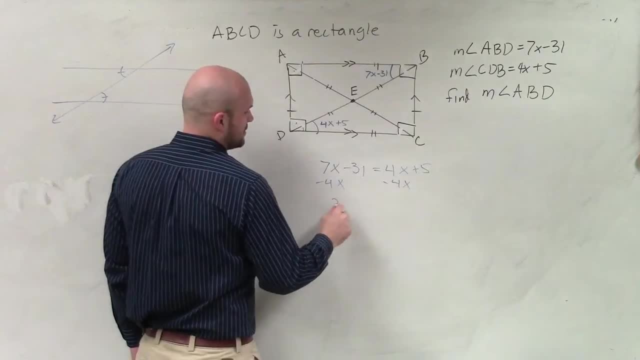 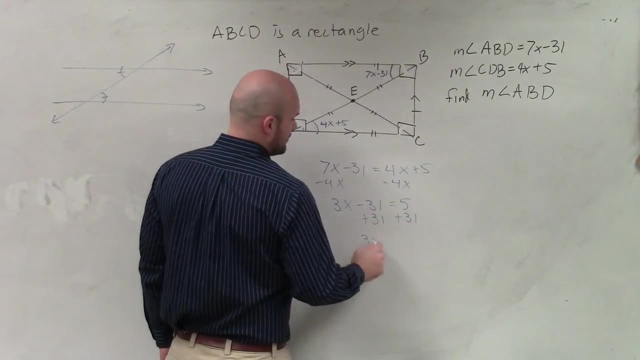 Now we can go and solve for X. So I subtract 4X on both sides: 3X minus 31 equals 5.. Add 31.. Add 31.. 3X equals 36.. Divide by 3.. 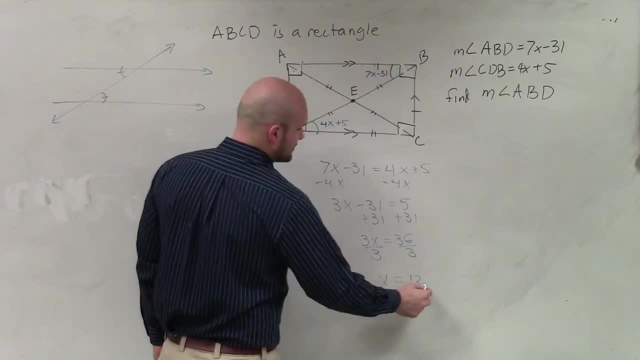 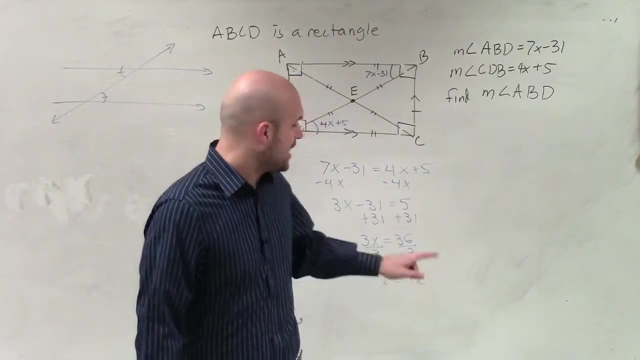 Divide by 3. X equals 12.. However, guys, that is not what the question is. The question does not say: what is X? So now what we need to do is take X and plug it into our value for our angle. 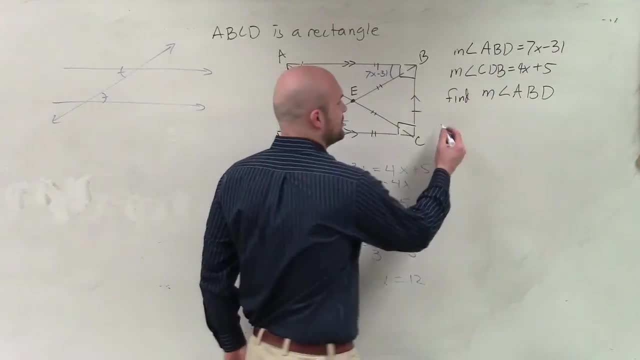 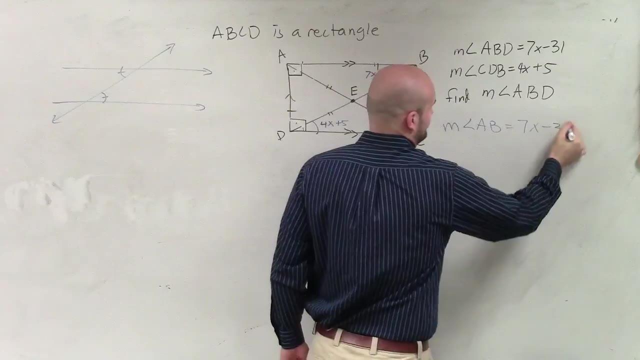 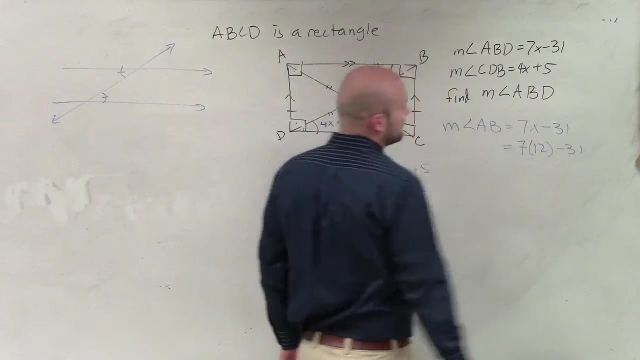 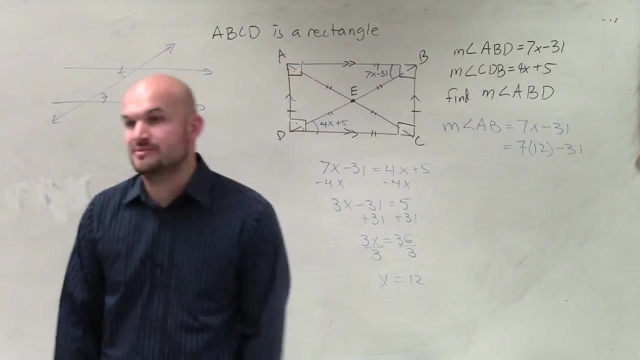 our measurement for our angle ABD, which is the expression 7X minus 31.. So the measure of angle ABD is 7X minus 31.. I now plug in X in for 12 minus 31.. And 5 times 12 is going to be 60..